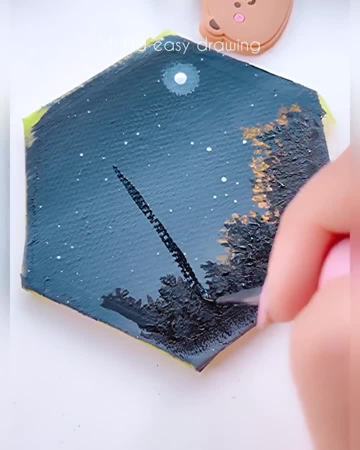 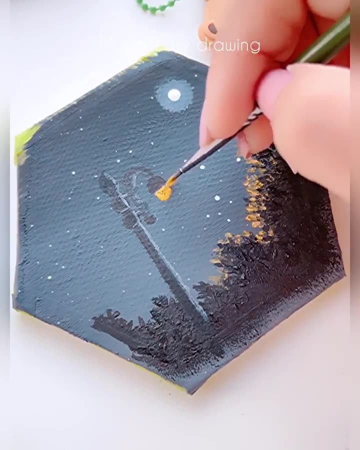 Is: let you know That when you touch my head, It all just goes away- The things I planned. to say, Oh baby. What I am trying to do Is let you know That when you touch my head, It all goes away: The things I planned, The things I would say. 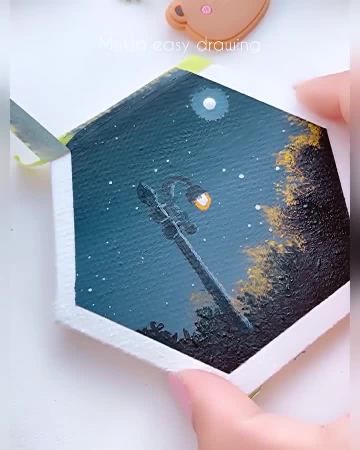 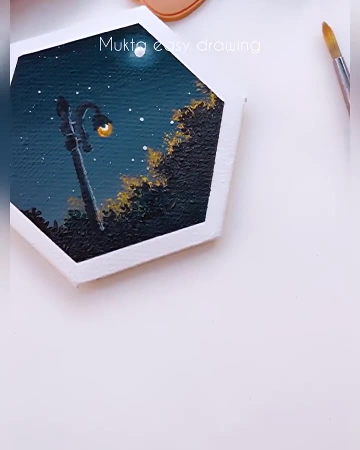 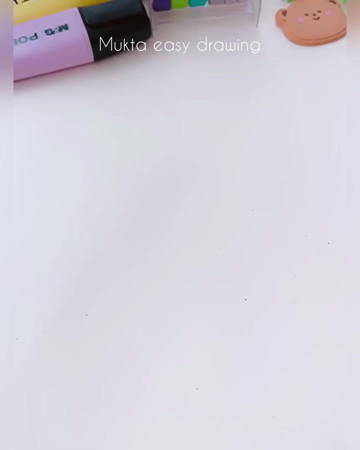 Now I keep rambling on. I sound so cliche. What I am trying to do Is say I love you And all the things that you do Sounds like a fool. What I am trying to do Is say I love you. I'm so in love with you. 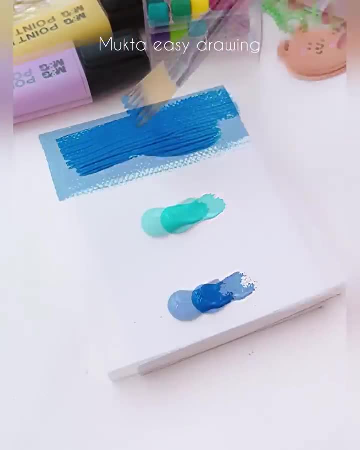 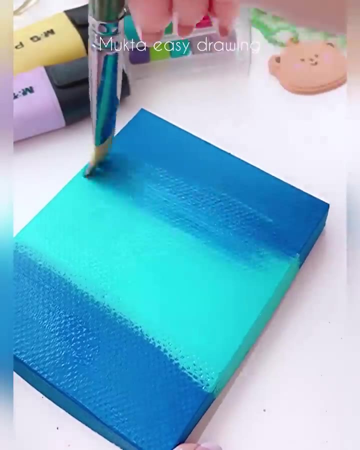 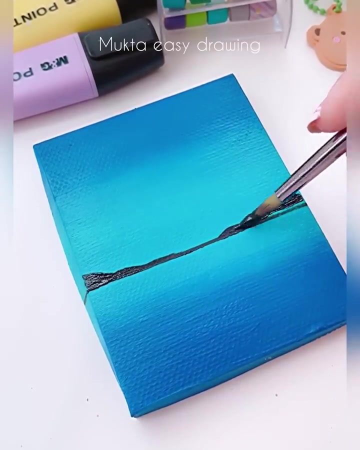 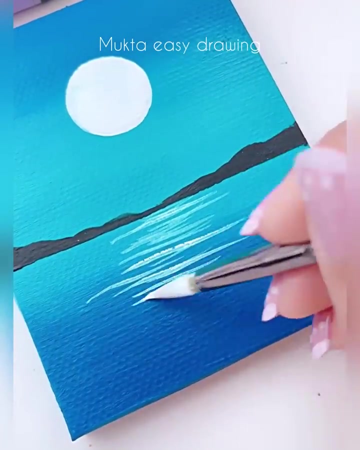 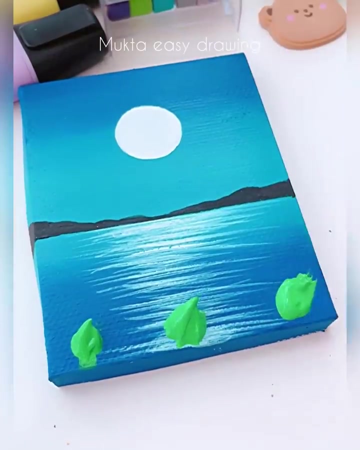 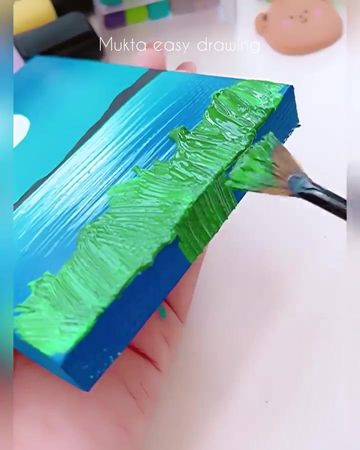 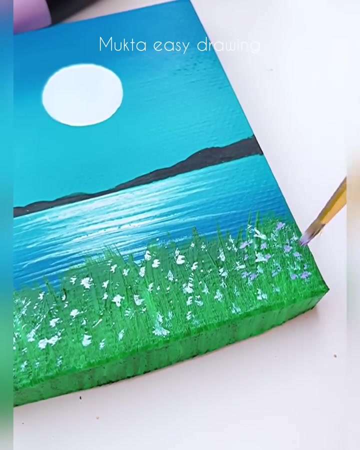 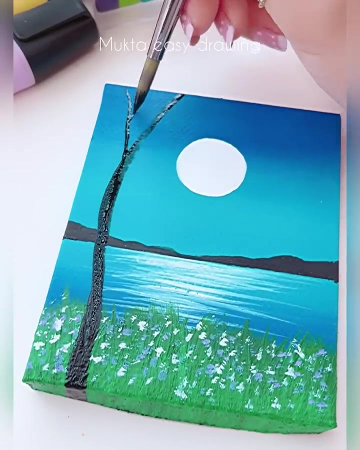 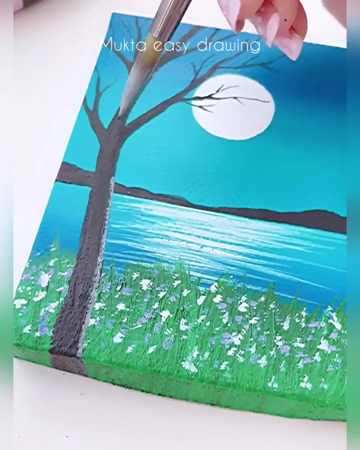 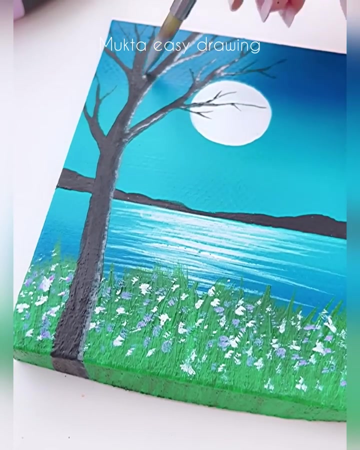 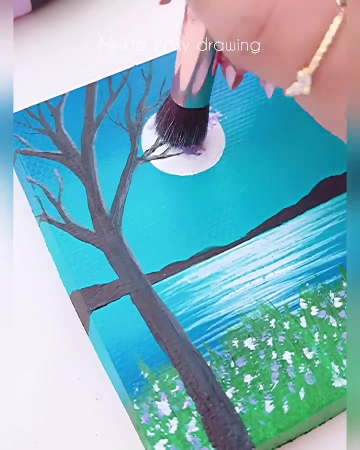 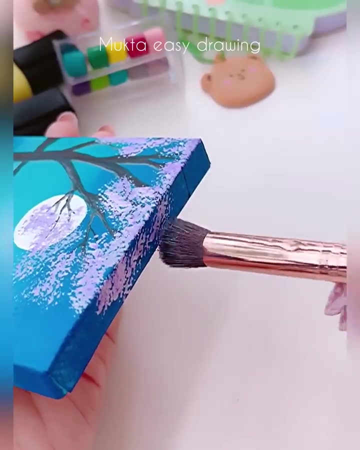 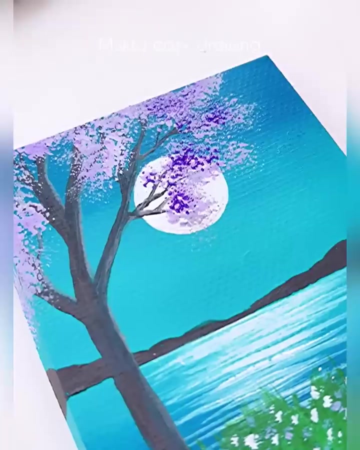 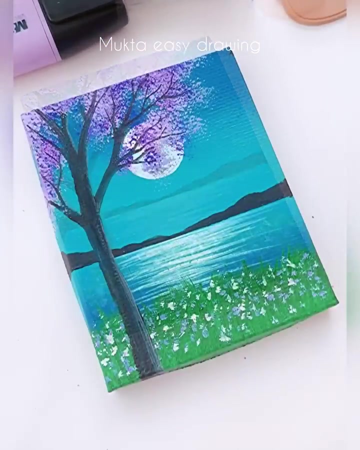 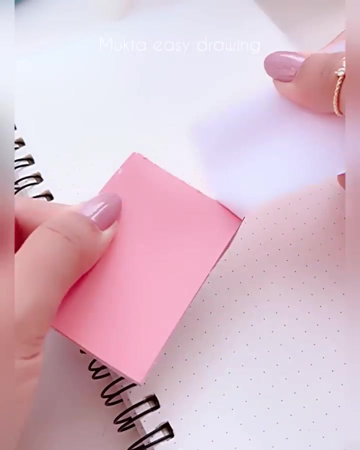 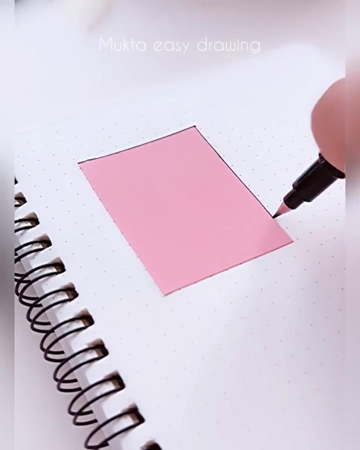 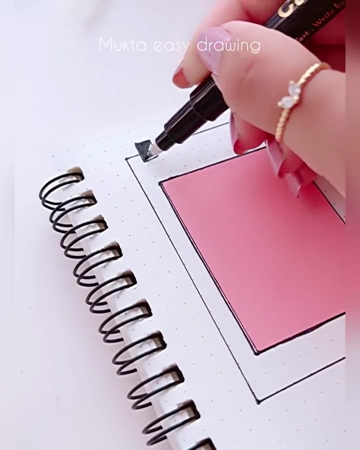 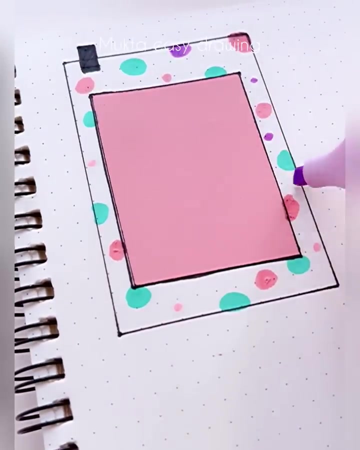 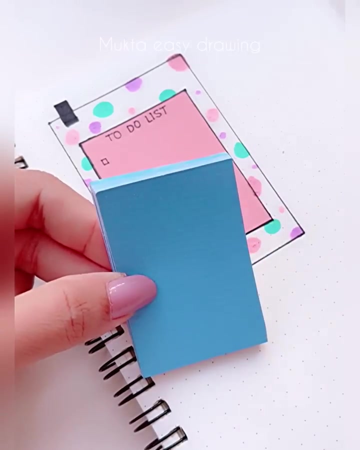 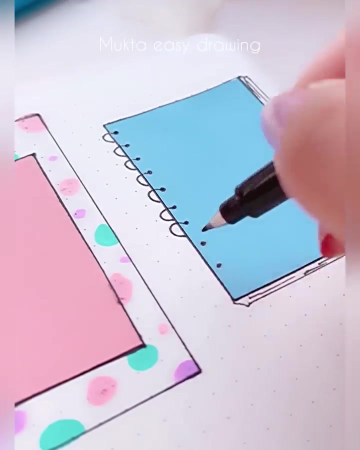 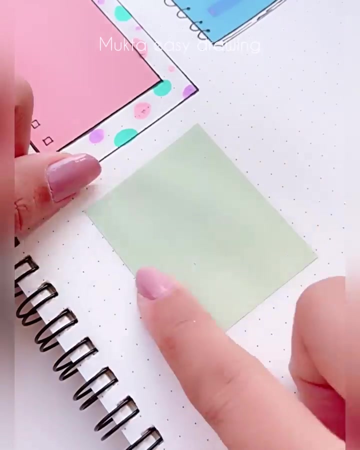 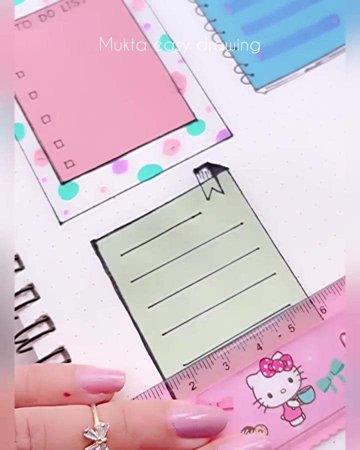 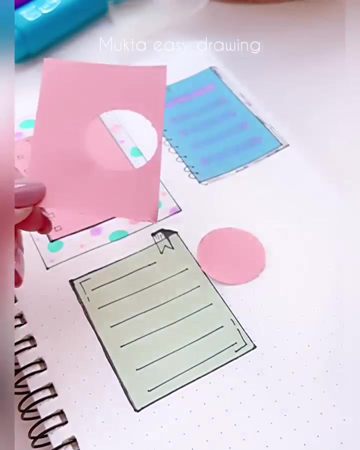 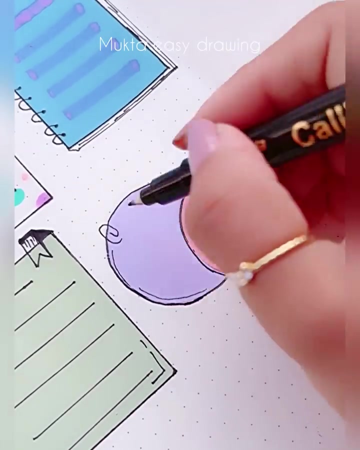 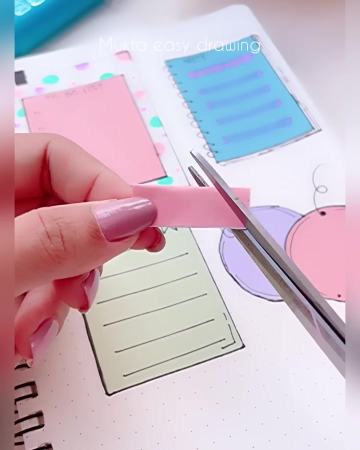 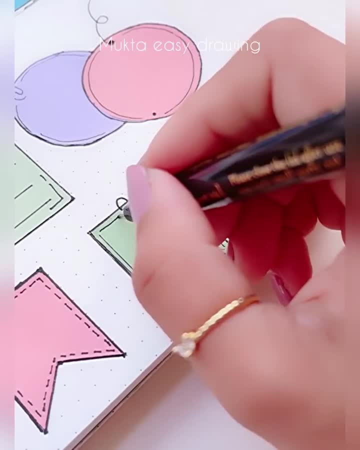 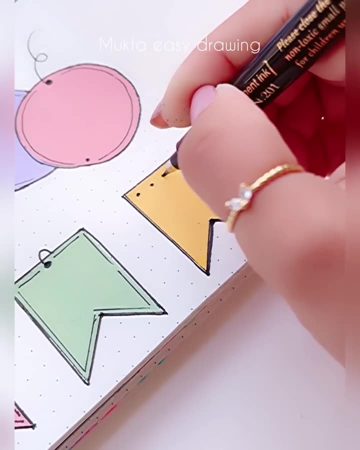 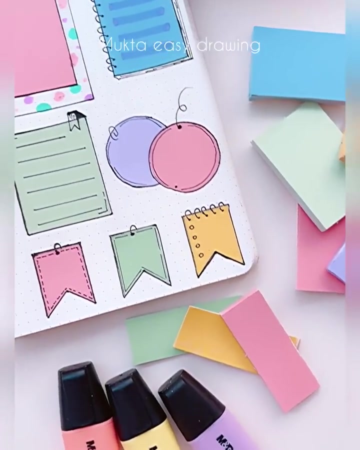 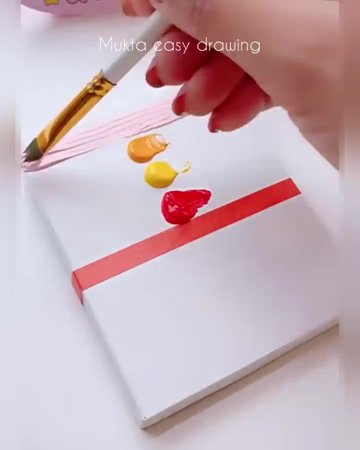 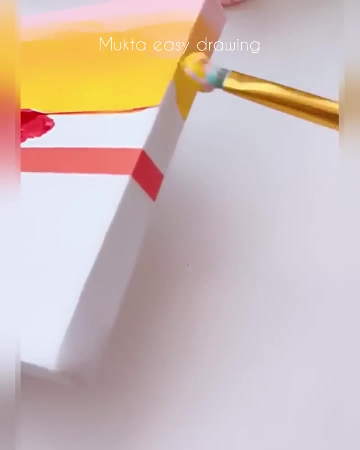 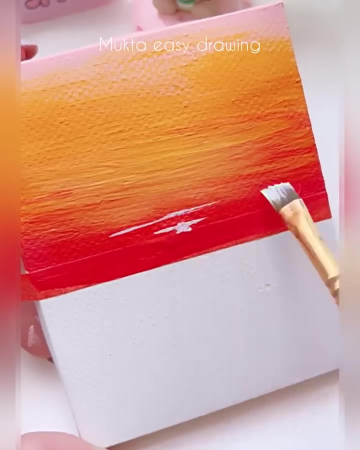 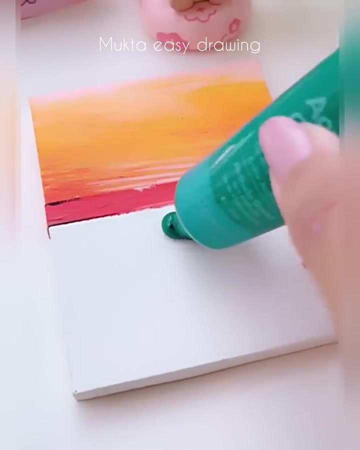 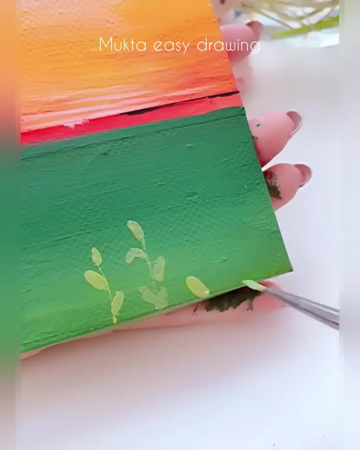 Is say: I love you, I put you on the back, We were talking, we were bad. Then you'd understand. You listened to all my problems. Your eyes would say: don't you worry, Kiss me on the cheek To make sure I was fine. Well, I'm not right now. 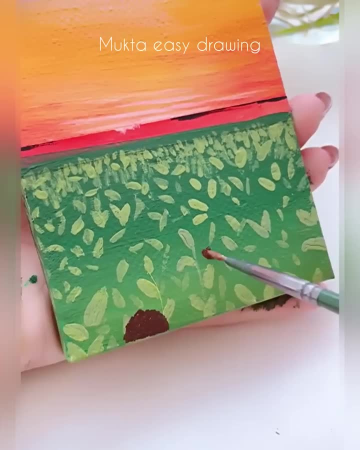 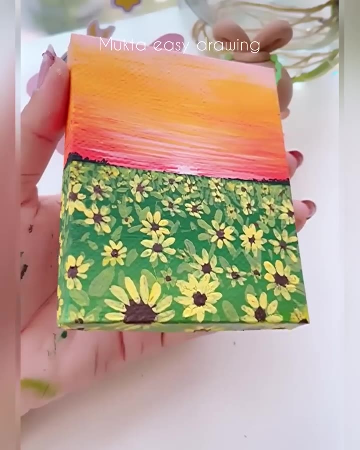 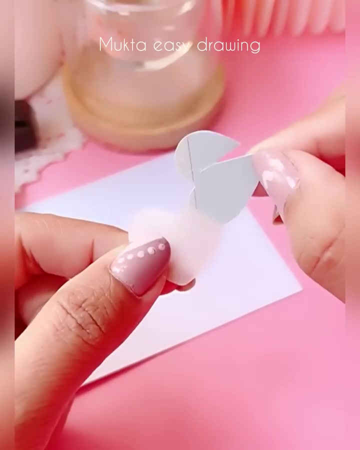 Cause I'm not good at what this says And my bad's barely around. I'm not good at what this says And I'm stuck in the middle All the time And my brother's gone to college, So we don't talk like before. I wish you were here. 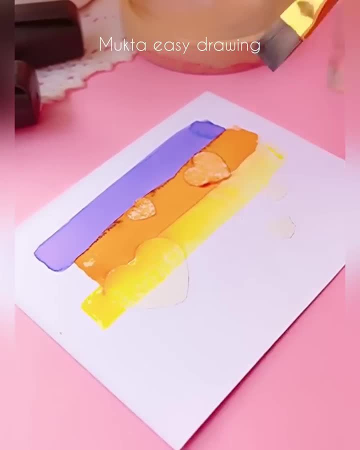 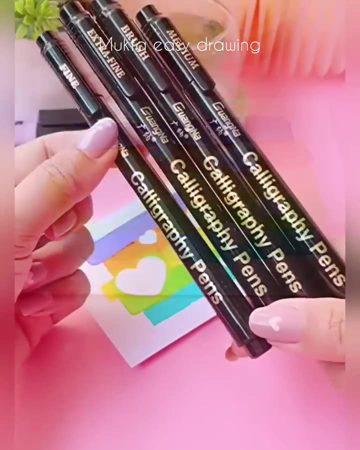 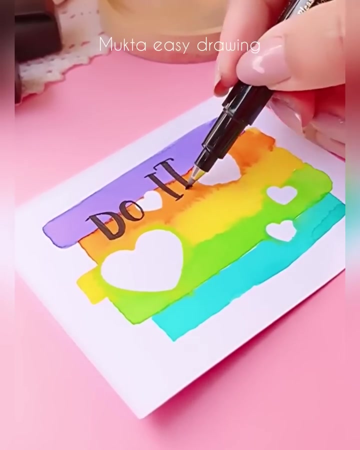 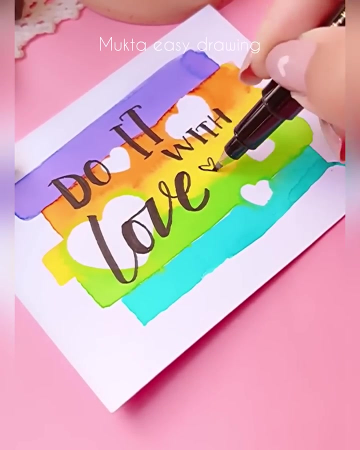 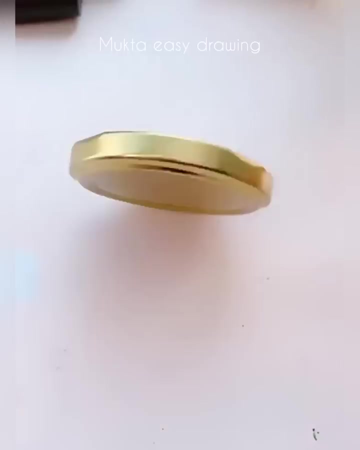 So I could tell you more, But you're not anymore. Walks in the carton, Secrets in the dark, Trips to the beach Basking in the sun Was your favorite thing. I hope that you do it still. You listened to all my problems. Your eyes would say: don't you worry. 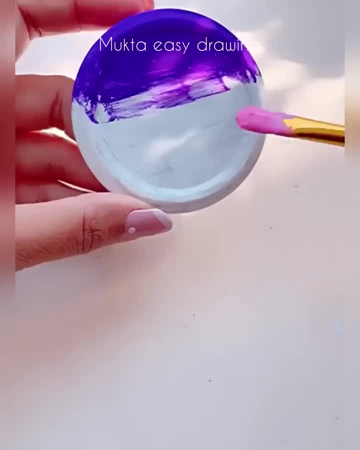 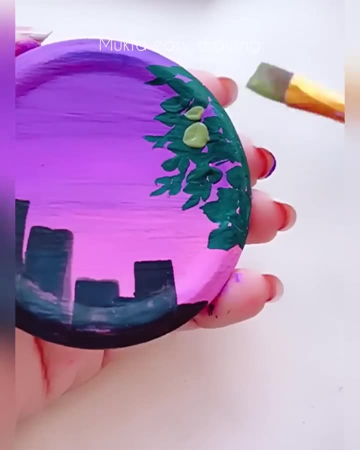 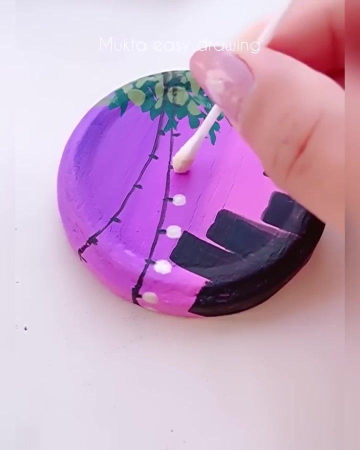 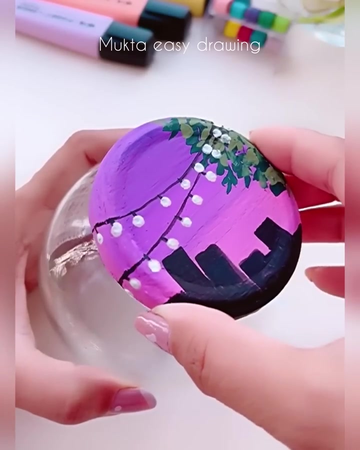 Kiss me on the cheek To make sure I was fine. Well, I'm not right now, Cause I'm not good at what this says And my bad's barely around And I'm stuck in the middle All the time And my brother's gone to college, So we don't talk like before. 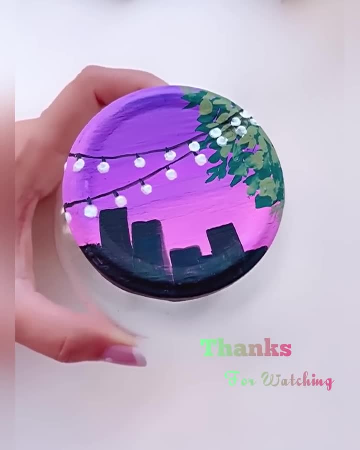 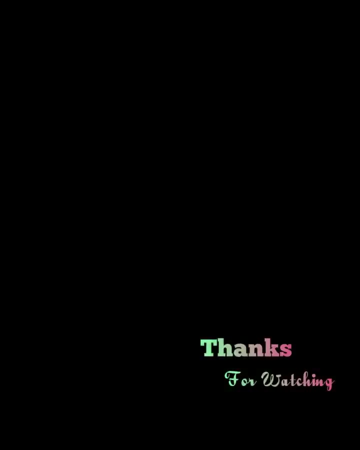 I wish you were here So I could tell you more. I wish you were here So I could tell you more, But you're not anymore.